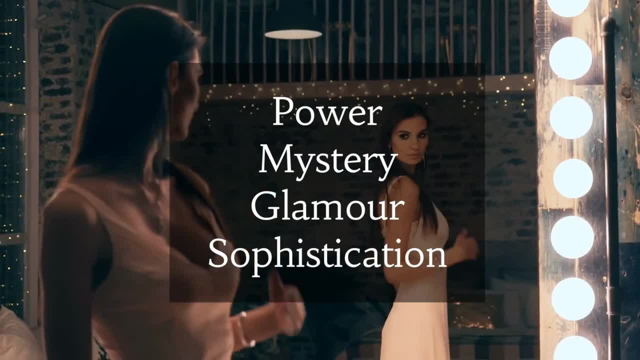 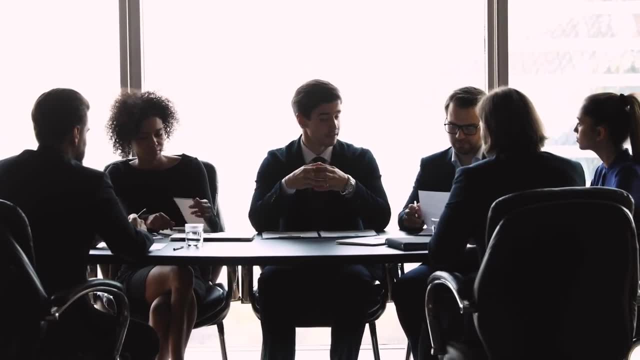 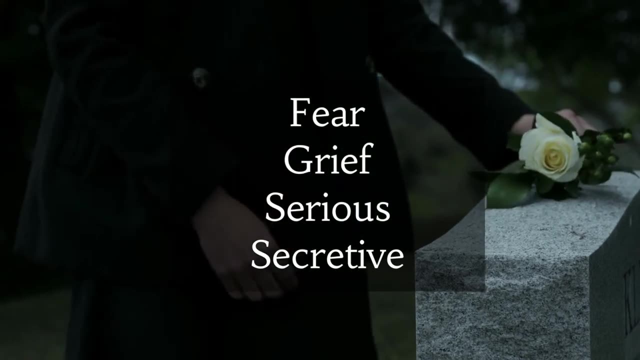 very classy color as well. The positive associations have to do with power, mystery, glamour and sophistication. Company logos that attempt to reflect those positive virtues are brands like Nike, Adidas and Adidas, Sony and even the New York Times. The negative associations of black have to do with things like 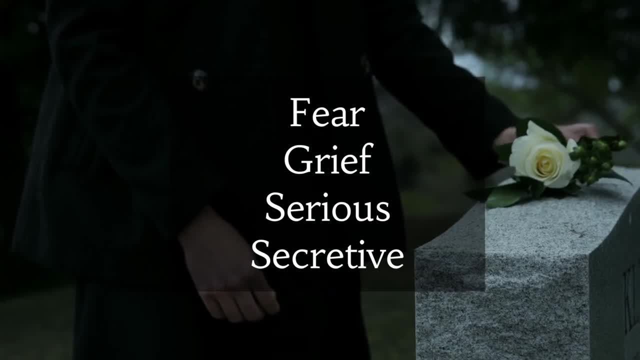 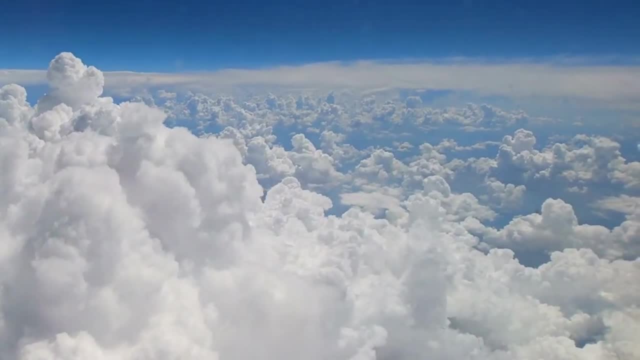 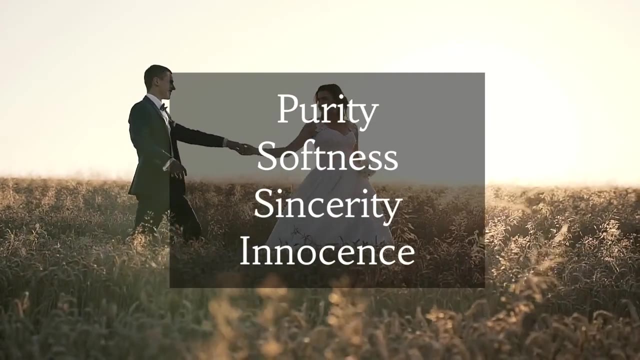 fear, grief, things being serious and secretive. White adds no extra visual weight and is often used as a supporting color. The positive associations of white are purity, softness, serenity and innocence. Negative associations of white have to do with things being plain. 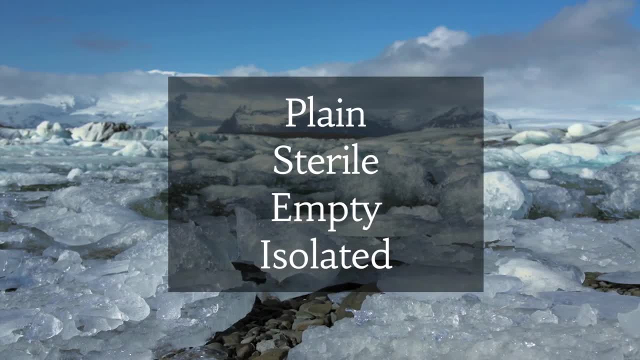 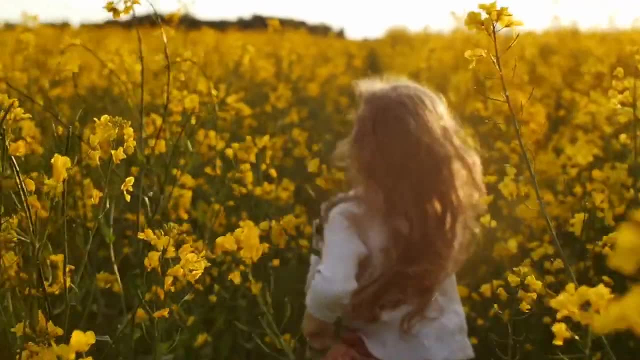 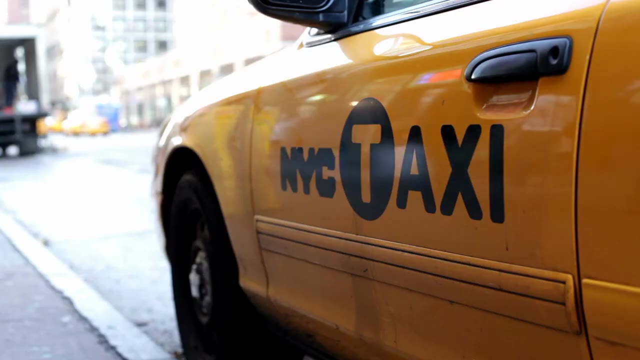 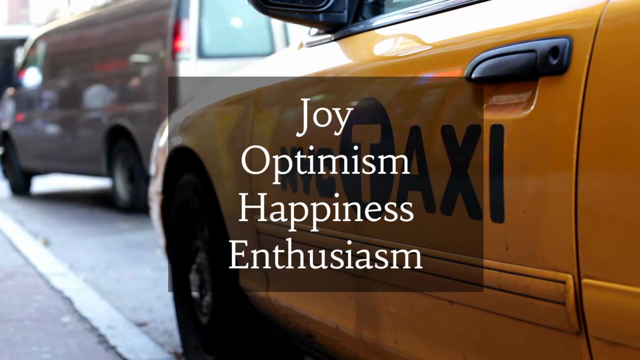 or sterile cold, even empty and isolated. Studies show that yellow releases serotonin, the happiness hormone. Yellow is very easy to see and it grabs our attention. hence the reason school buses and taxis over in America are yellow. The positive associations of yellow are things like joy, optimism, happiness, enthusiasm. 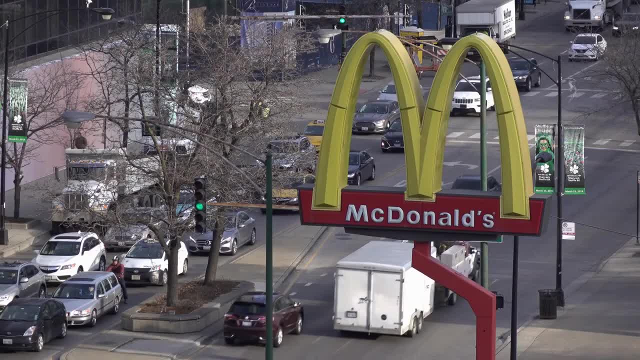 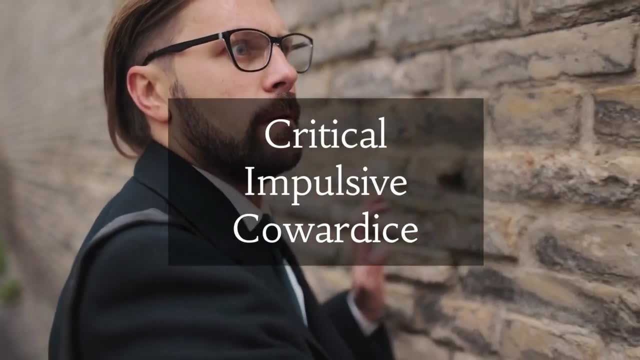 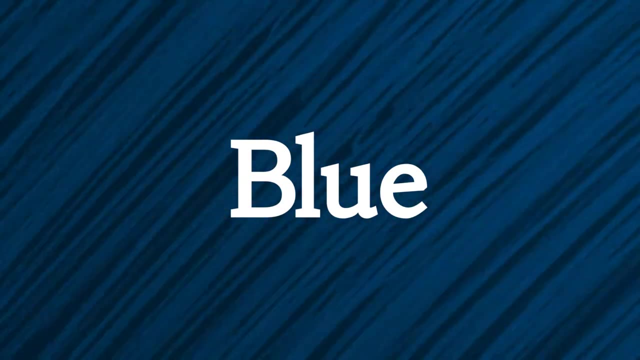 Company logos that try to incorporate some of those positive things of yellow are brands like McDonald's, Chubba Chubs, Snapchat and the Commonwealth Bank. The negative associations of yellow are being critical, impulsive and cowardice. Blue is reportedly the world's most common favorite color. We associate it with the sky and water. 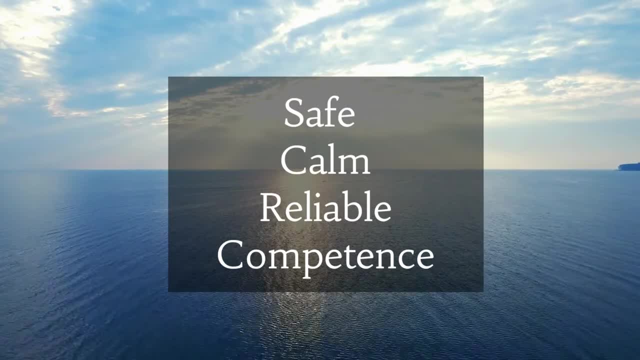 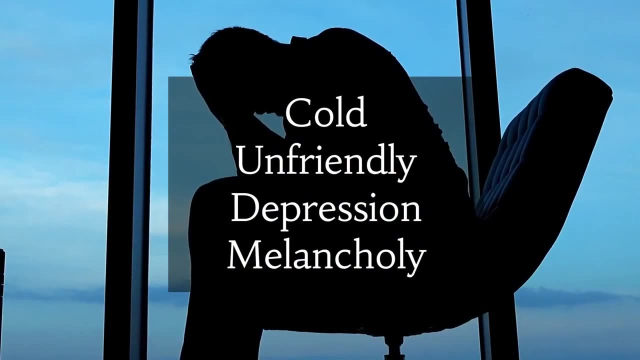 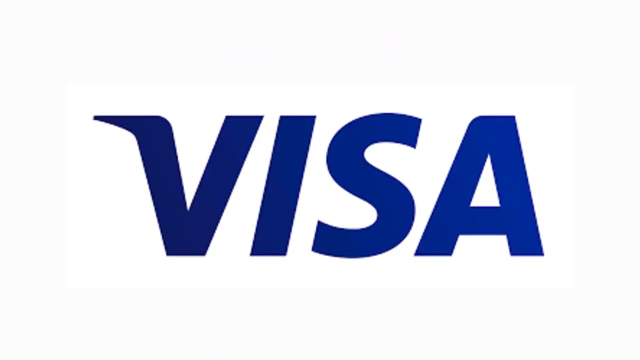 The positive associations of blue are being safe, calm, reliable competence. The negative associations of blue are cold, unfriendly, depression, melancholy. It should come as no surprise that many social media companies, tech companies and financial institutions choose the color blue in their company's logo. 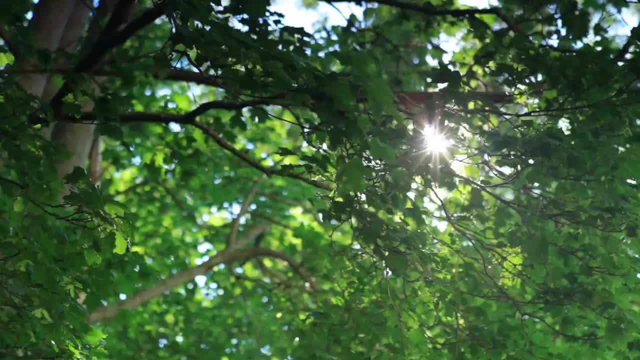 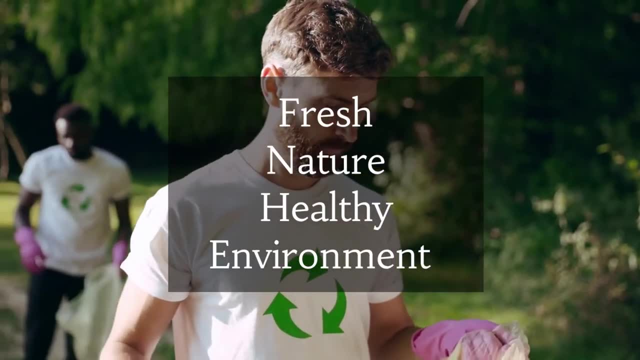 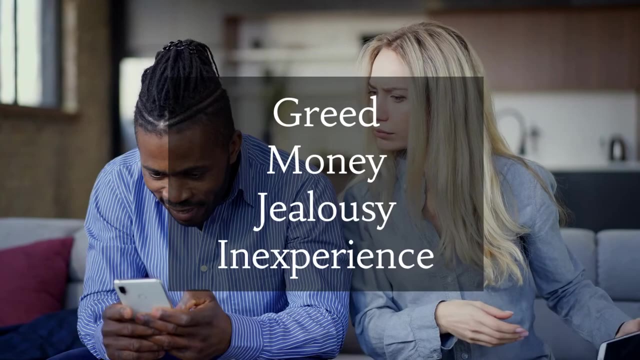 Green is the easiest color for the eye to process. We associate green with being fresh, nature, healthy and the environment. The negative associations of green have to do with greed, money, jealousy and inexperience. Shakespeare calls jealousy the green-eyed monster. 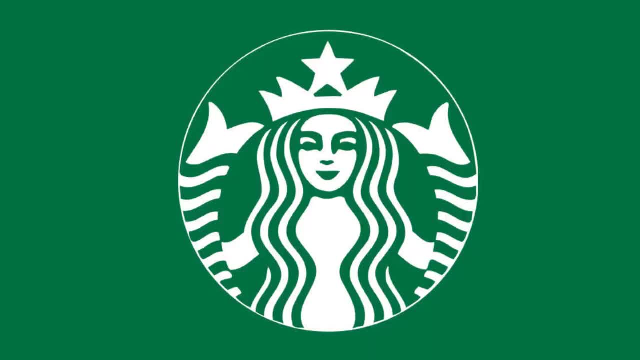 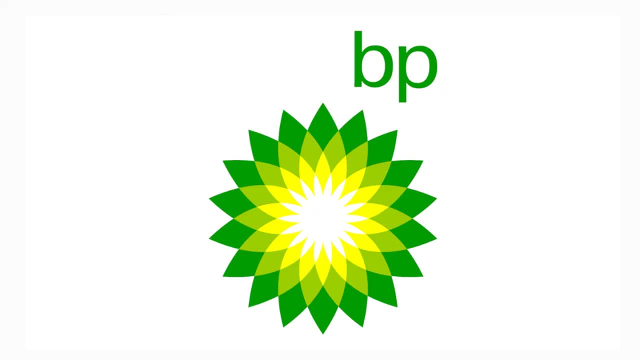 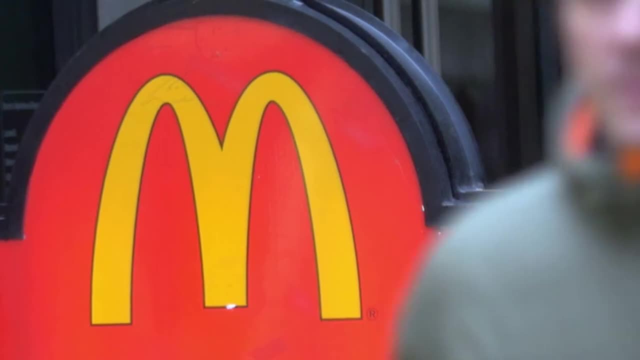 monster companies that use the color green in their logo are attempting to reflect those positive virtues of being environmentally friendly and healthy. you know, like BP, the oil and gas giant, studies have shown that the color red raises the heart rate and also increases appetite. it should come as no surprise that many fast food chains use red in. 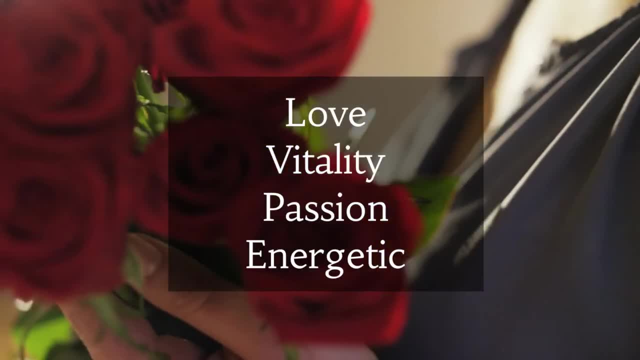 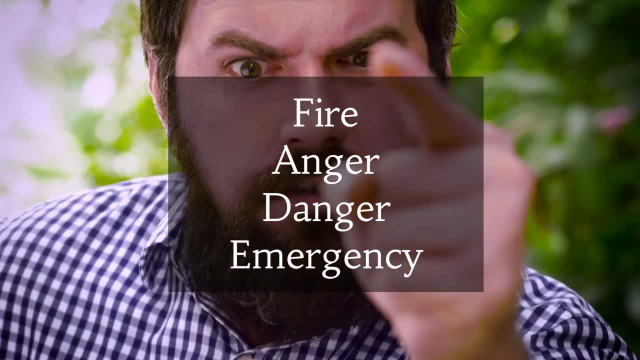 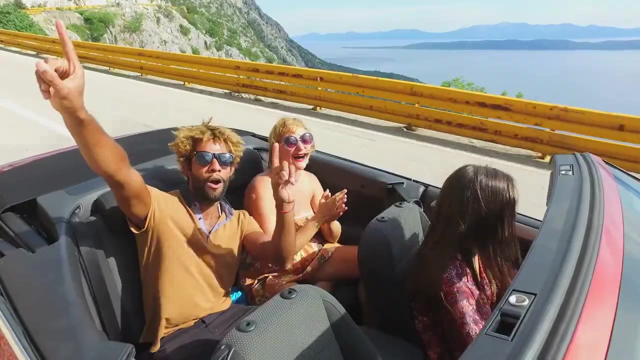 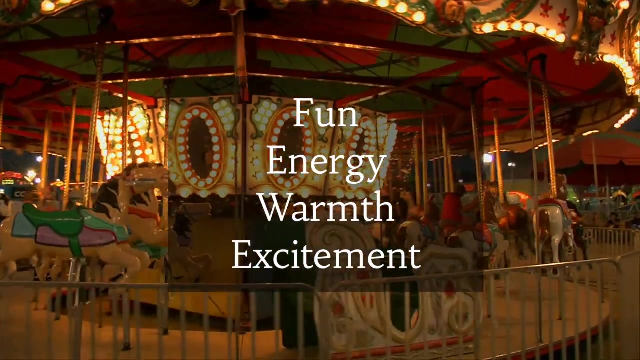 their advertisement. the positive associations of the color red are love, vitality, passion, being energetic. the negative associations of the color red have to do with fire, anger, danger and emergency. oranges are bright attention, getting color. it's a perfect call to action. the positive associations of orange have to do with being fun. there's energy. 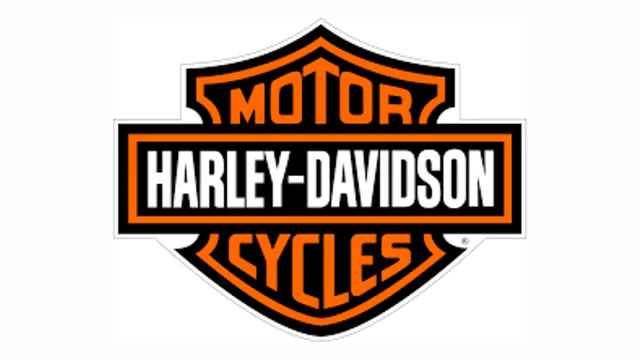 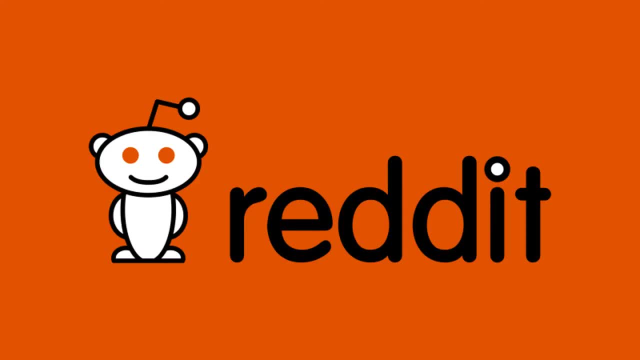 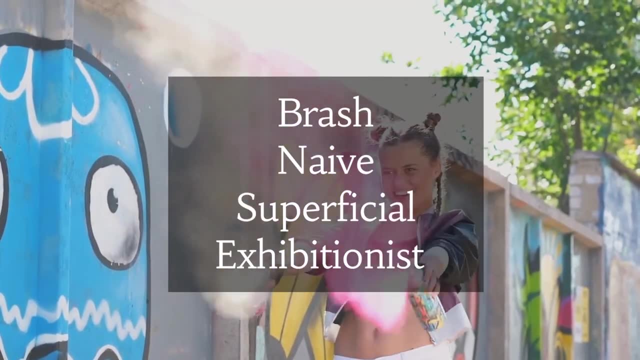 involved, there's warmth and excitement. company logos that use the color orange attempt to reflect those positive virtues of fun and energy. energy and excitement, like Fanta, Reddit and Nickelodeon. However, the negative associations are being brash, naive, superficial or an exhibitionist. 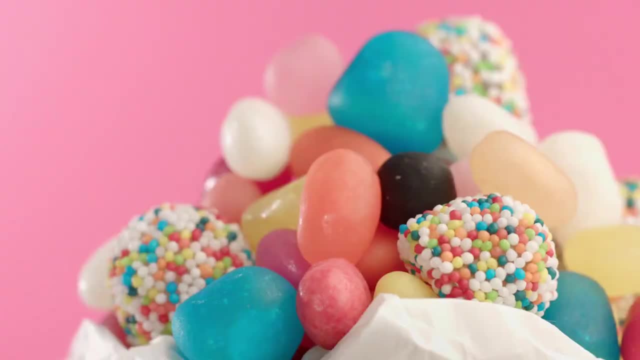 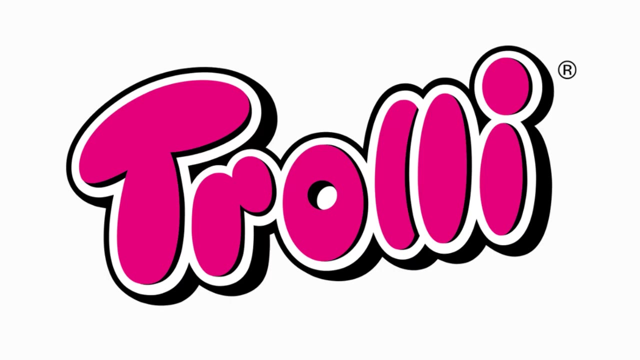 In Japan, pink is associated with spring due to the cherry blossoms. Sweet, young, kindness and feminine are the positive associations of pink. Logos that use pink include brands like Trolley, Baskin, Robbins, Barbies, Cosmopolitan and. 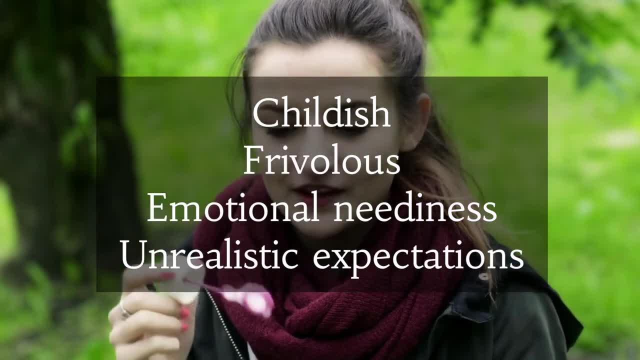 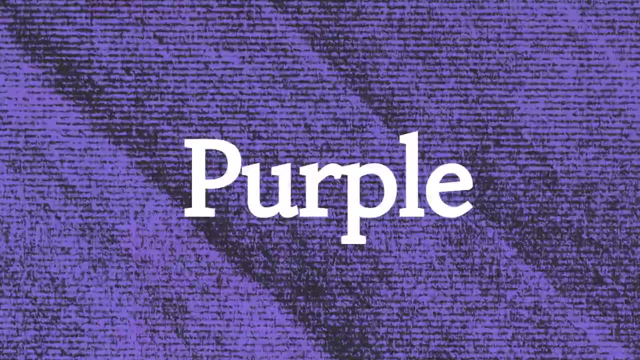 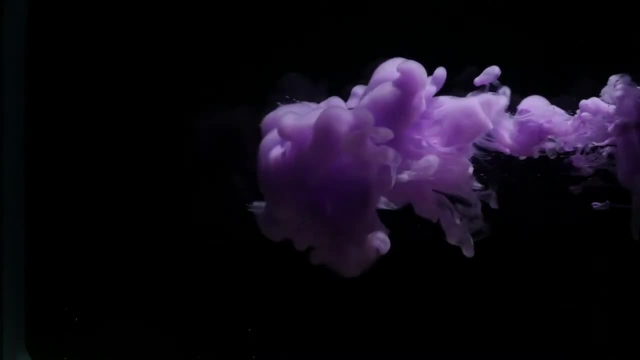 Victoria's Secrets. Childish, frivolous, emotional neediness and unrealistic expectations are associated with pink. The colour purple has been shown to stimulate problem solving. Historically, it was also the most expensive and complex colour to produce, as it was made from the mucus of sea snails. 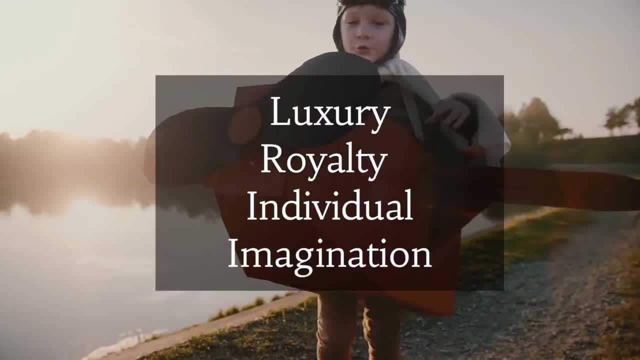 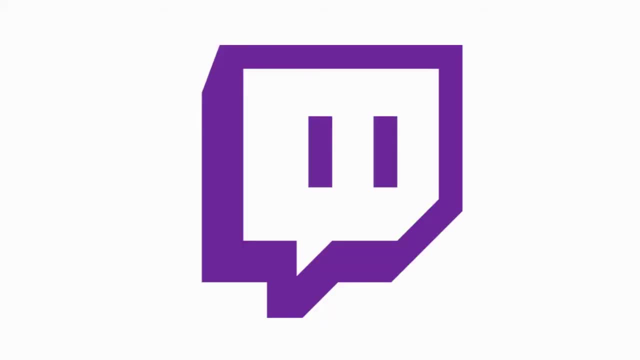 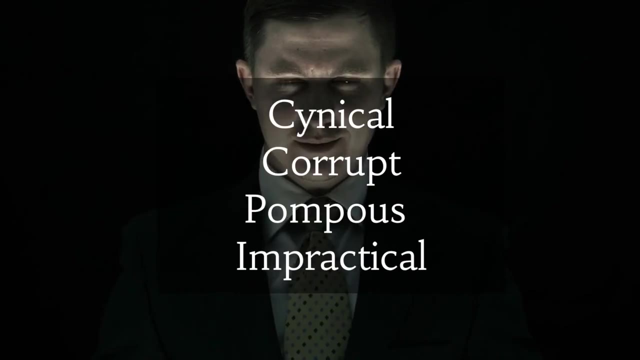 Which is why it has been linked with luxury. We also associate it with being an individual and the imagination. Cadbury, Taco Bell, Twitch and the Starlight Children's Foundation all use the colour purple in their logos. The negative connotations of purple have to do with being cynical, corrupt, pompous and 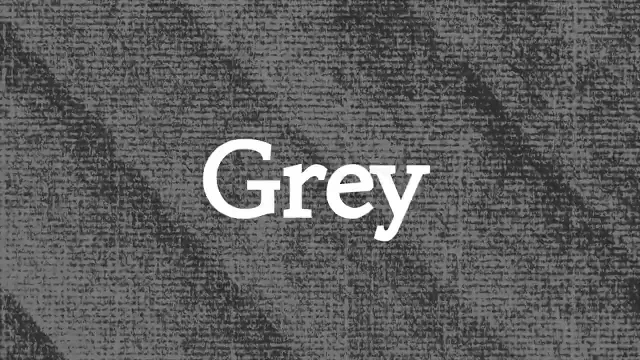 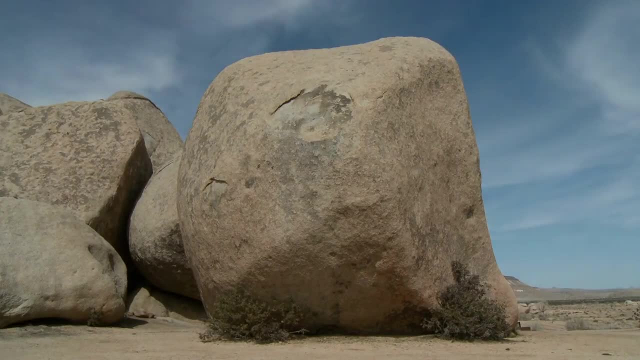 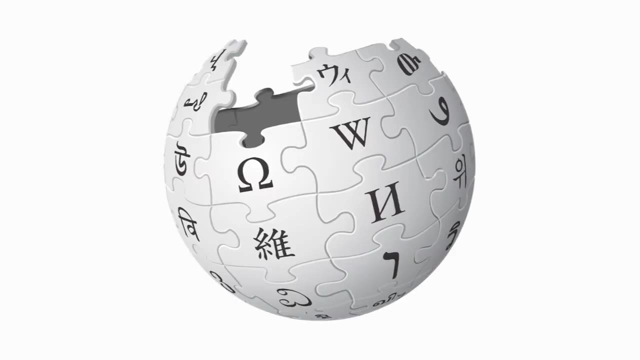 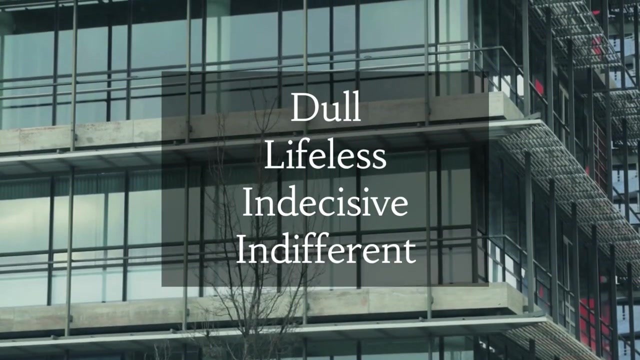 impractical. Grey is associated with rocks and stones, sturdiness and longevity. It is a timeless colour. Grey implies something being solid, neutral. corporate and professional Grey logos want to appear impartial and timeless. The negative associations of grey are dull, lifeless, indecisive and indifferent. 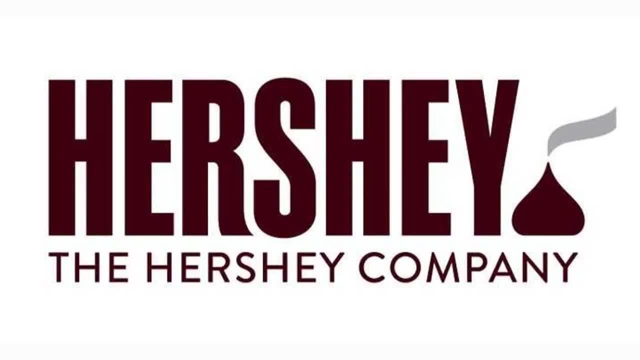 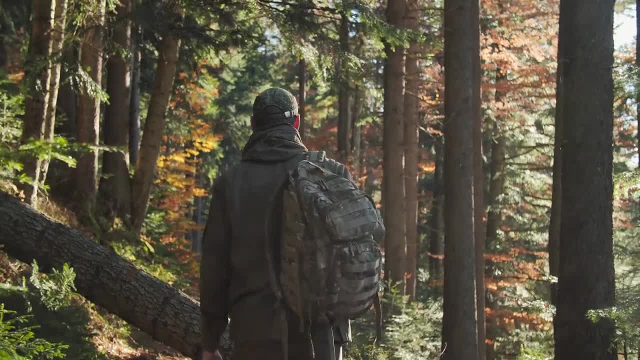 The first thing that comes to mind when we think of brown are probably things like chocolate and coffee. Brown is a natural and earthy colour And, if done right, can be very soothing. Brown is a natural and earthy colour And, if done right, can be very soothing.